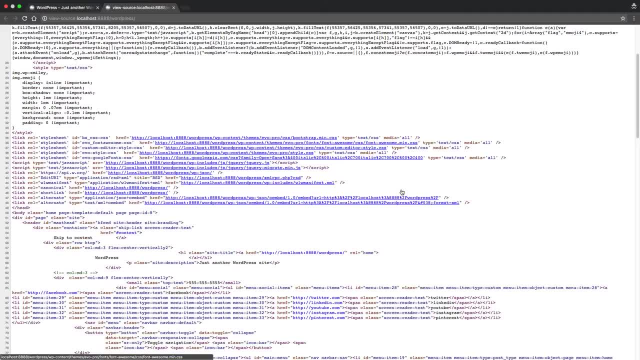 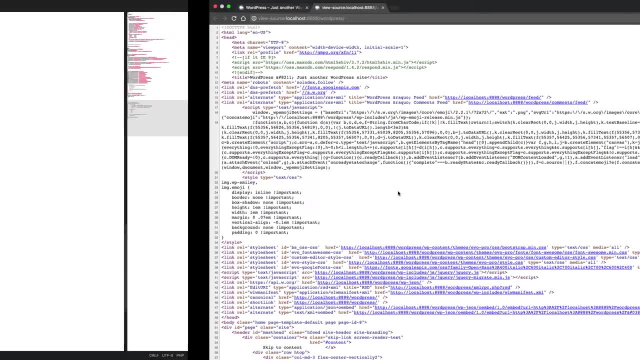 page source. So we're here viewing the source of a local website on my local server, and you see that the HTML is not minified. All right, so now, if you want to minify it, I have the snippet of code right here. I'm going to uncomment that out. 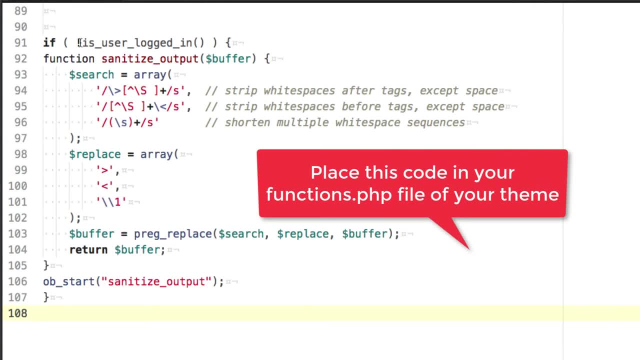 I'm going to save it and let's walk through this real quick. First, there's an if conditional statement. There's checking to see if the user is logged in, and if they're not logged in, then we're going to run this code here. It's going to run the. we're creating a function: sanitize output. 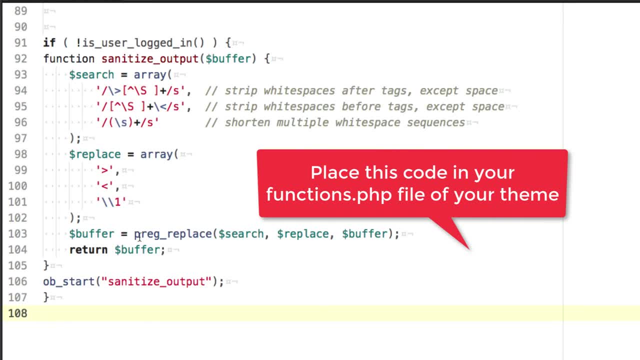 with the buffer variable and we're creating three variables inside of there. and then, inside these first two variables, we have arrays and inside those arrays we have these elements here and you can see right here that the HTML is not minified. So I'm going to save it and let's walk through this. 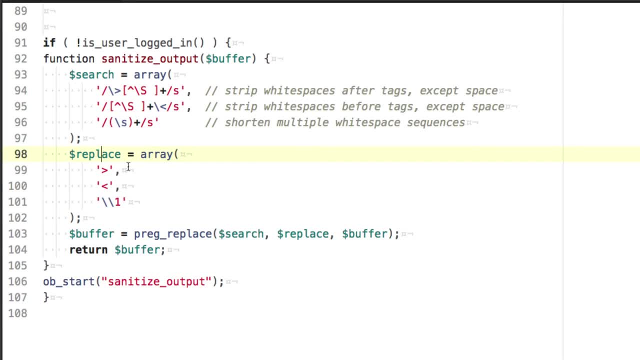 here what they're doing: In the replace array, we're replacing it with these items here and then in the final variable we're using the correct replace function. and then we're taking the items in the search array, replacing it with the items in the replace array and we're holding it inside the 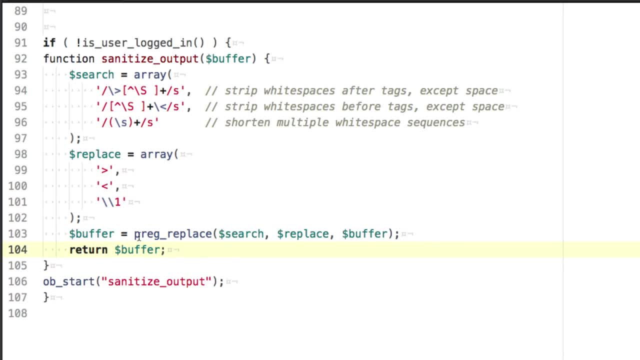 buffer variable and then we're going to return the buffer variable and then we're going to close off that function and then we're going to underscore start And then sanitize output, which is the name of our function up here, and then we're going to close out this whole. 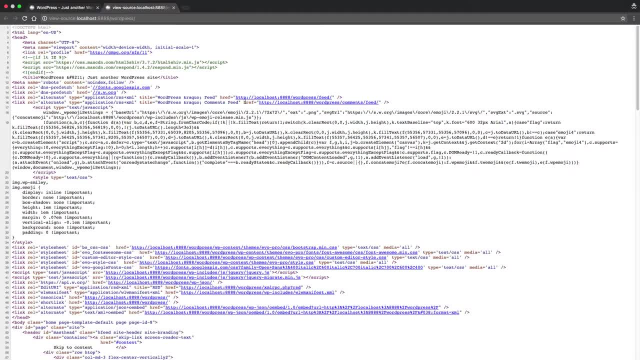 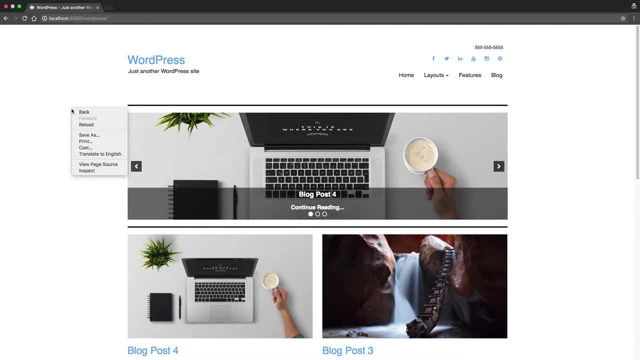 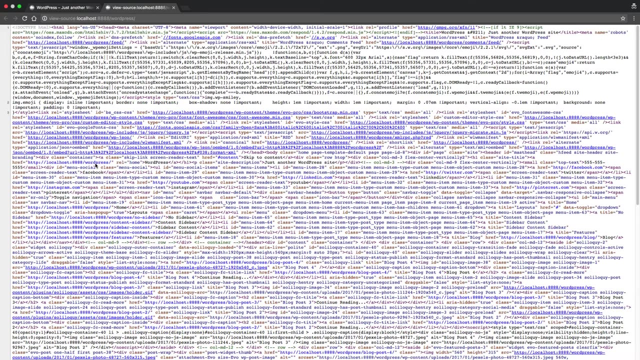 entire if conditional. So now that we did this, you remember it was not minimized. Let's close this off. Refresh this. We're going to view page source again and now it's completely minified and this is only going to happen if the user is not logged in. This is a great way to minify the code of your. 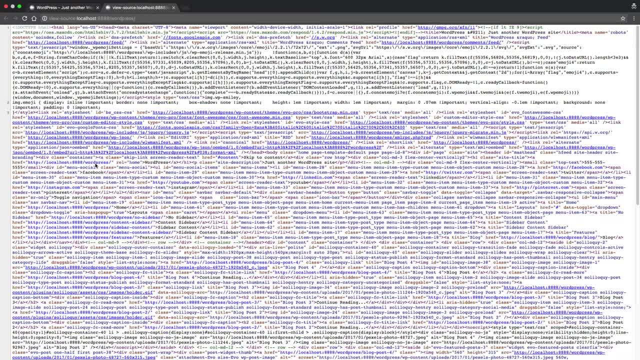 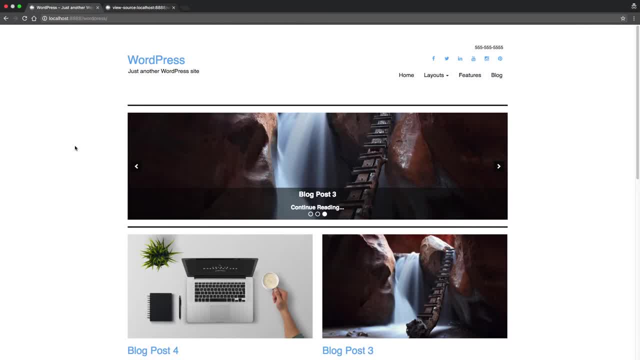 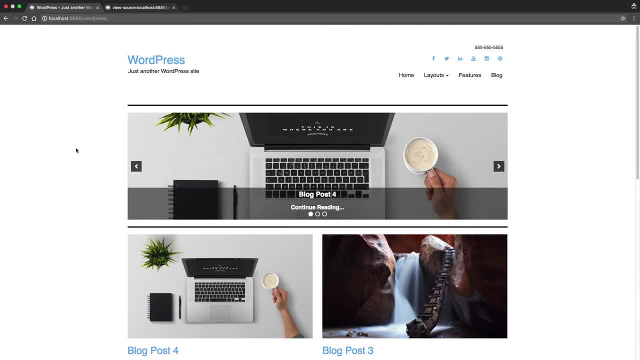 web pages and website and also it helps to benefit in terms of the page load times and that is an SEO ranking factor. So I definitely think that we should always try to find every single possible way, you know, to minify the amount of code that we can and to minimize the amount of time it takes for a web page or 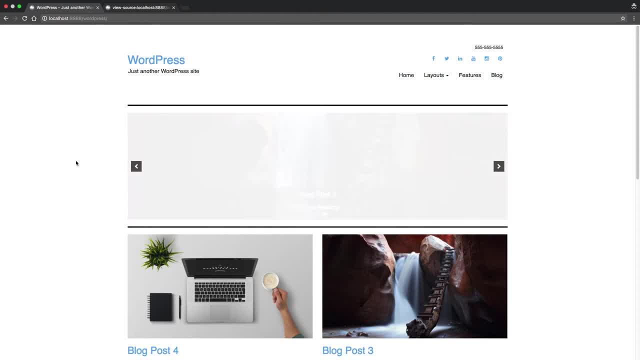 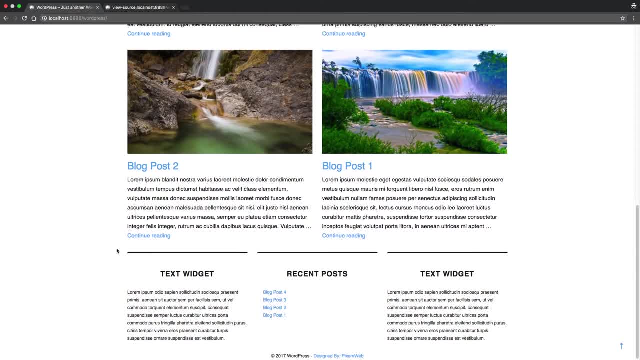 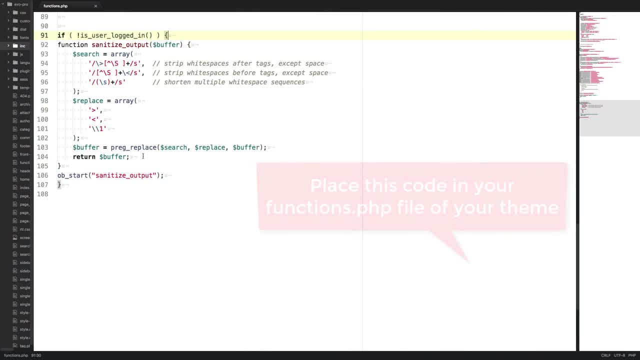 of the code is one of them, and this snippet of code here is what you can use to to minify your code. Now, again, this is only for advanced users, but it does work and I'd always recommend that people test it out in their local environment. 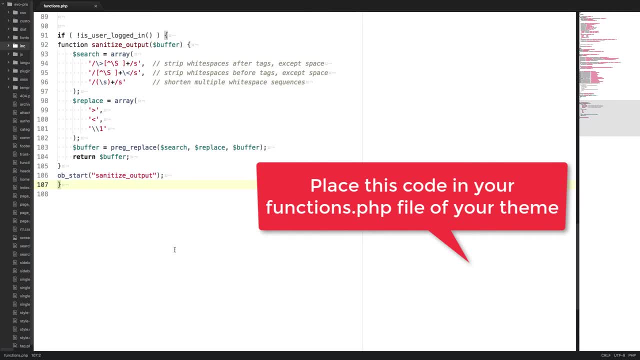 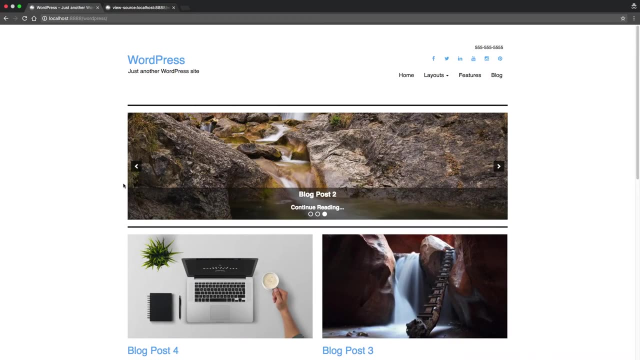 first and then, if they're satisfied, then they can try it out on their production site. always take a backup of your database. take a backup of your files, just in case you have to revert to them. you know, sometimes adding custom code can cause a conflict with a plug-in that you're using or the theme that you're using you. 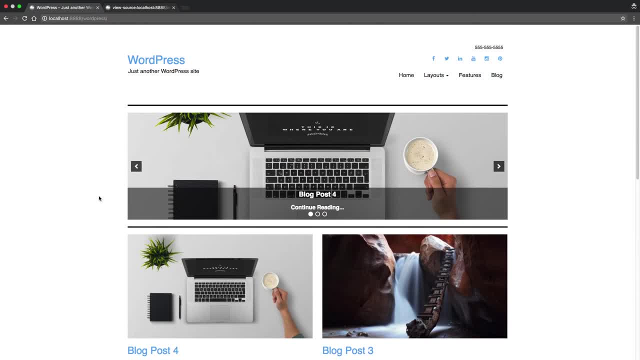 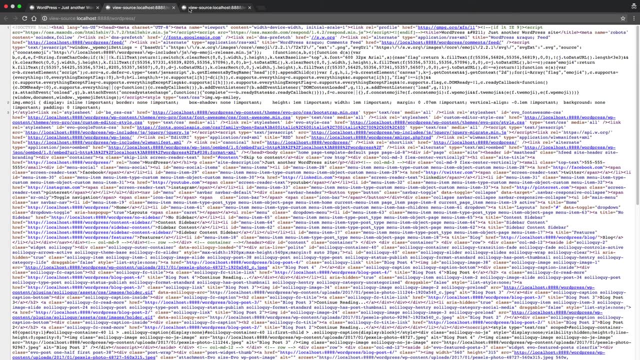 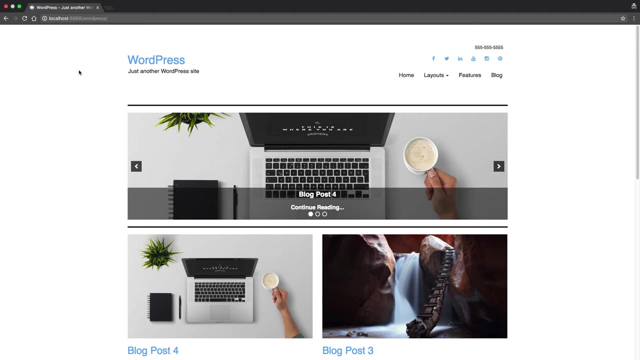 know if there's a. you know potentially something more with the code or something like that, all right, but this code is clean, it works, it shows you the generated output is minified and this will help you with the page load time of your website and that should help you within, you know, with one of the many 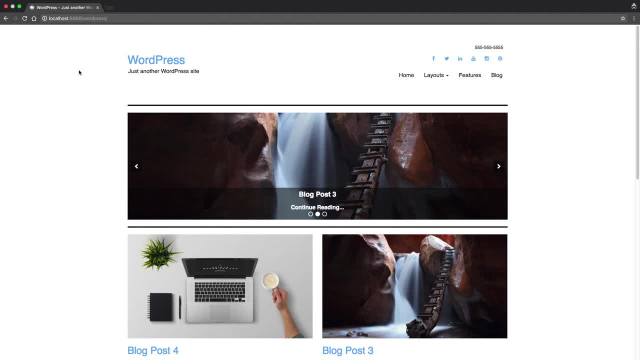 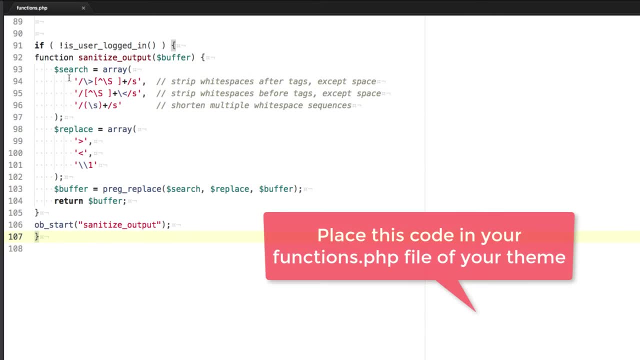 ranking factors that Google uses to determine who ends up on page one. all right, hopefully you found this episode helpful. just to recap, just provided a snippet of code that you can use on your website. and what this does? it strips out the white space after tags and white space before tags and shortens the 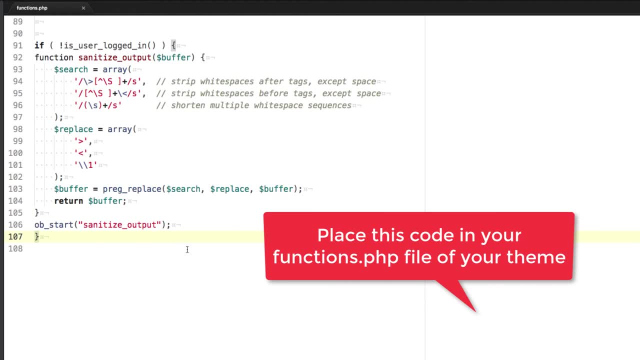 multiple white space sequences and it's a snippet of code that does, you know, a lot of work for you, and that's what we're going to talk about today. you know what a lot of plugins do, but this does it in. you know, just a few lines. 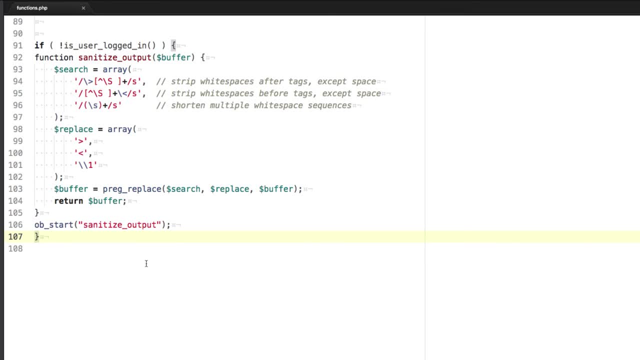 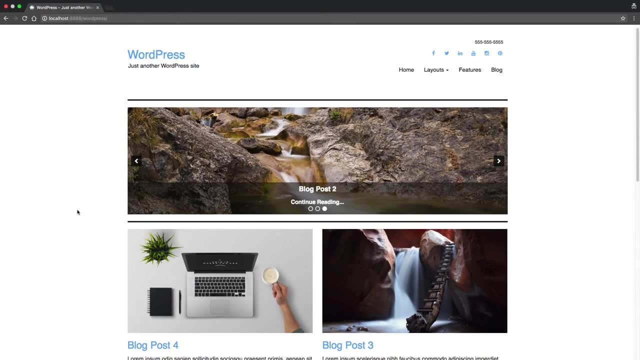 of code right here, very simple to do, all right. hopefully you enjoyed this video where we I showed you how to minify your HTML code. if you did, give us a thumbs up and don't forget to subscribe, because I'll show you more ways that you can. 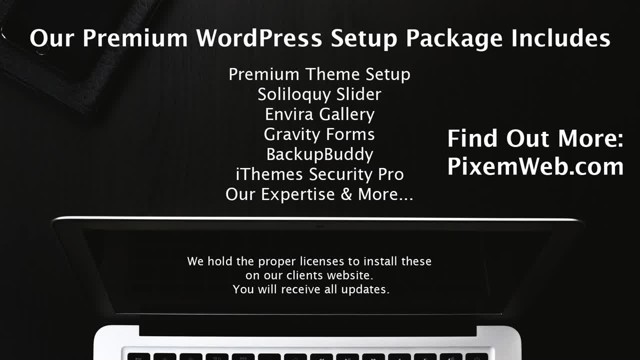 optimize your website for peak performance, for search engine optimization and, most importantly, for user experience. all right, again, thumbs up and don't forget to subscribe. I'll see you next time.